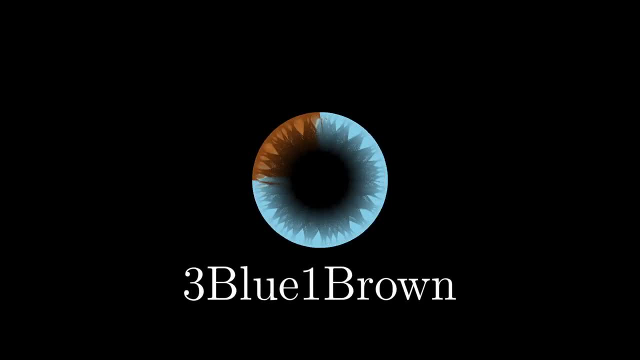 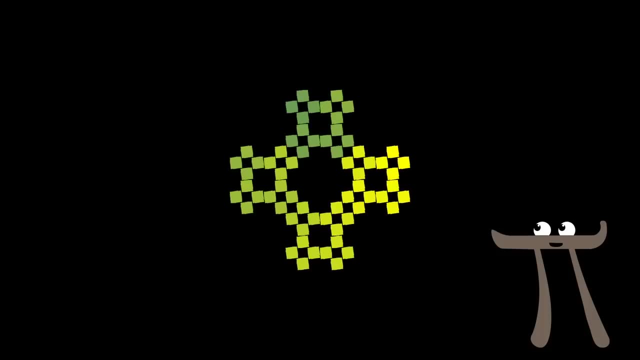 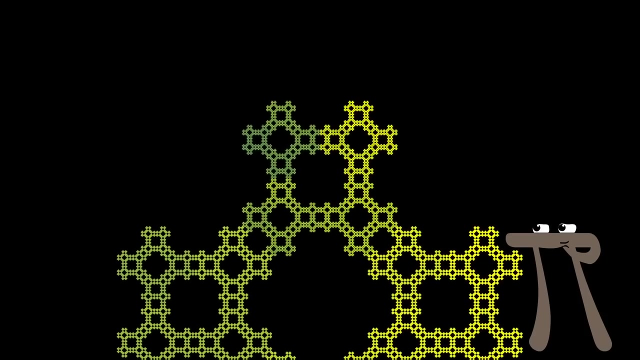 Who doesn't like fractals? They're a beautiful blend of simplicity and complexity, often including these infinitely repeating patterns. Programmers in particular tend to be especially fond of them because it takes a shockingly small amount of code to produce images that are way more intricate than any human hand ever could hope to draw. But a lot of people. 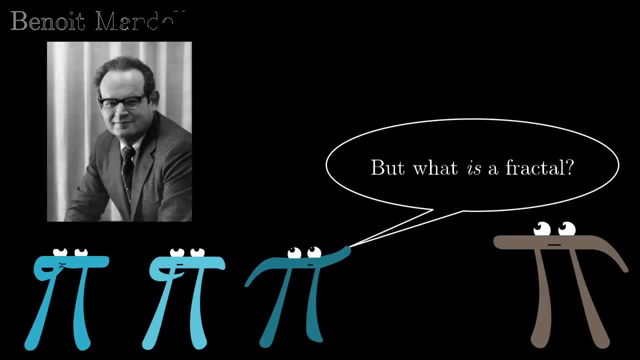 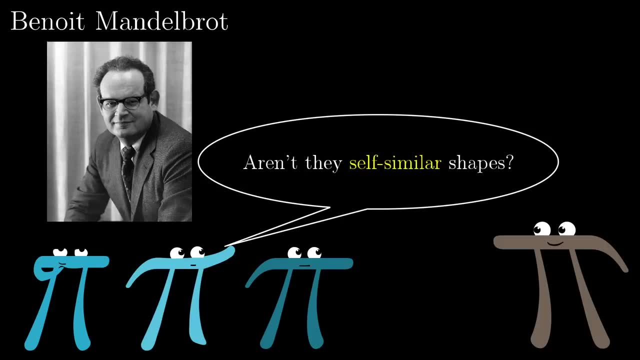 don't actually know the definition of a fractal, at least not the one that Benoit Mandelbrot, the father of fractal geometry, had in mind. A common misconception is that fractals are shapes that are perfectly self-similar, For example, this snowflake-looking shape right. 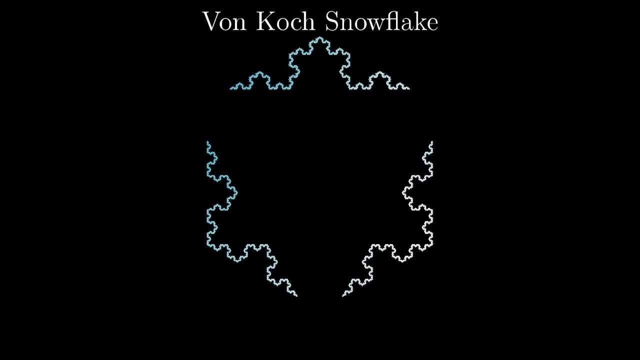 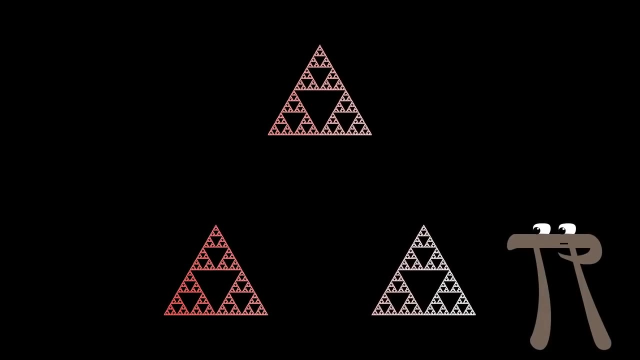 here called the Van Gogh snowflake, consists of three different segments, And each one of these is perfectly self-similar in that when you zoom in on it, you get a perfectly identical copy of the original. Likewise, the famous Sierpinski triangle consists of three smaller, identical copies of itself. 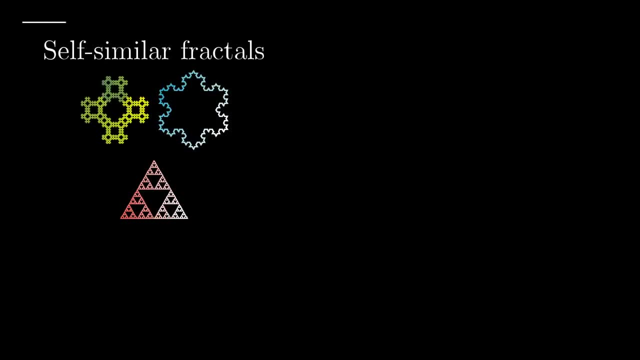 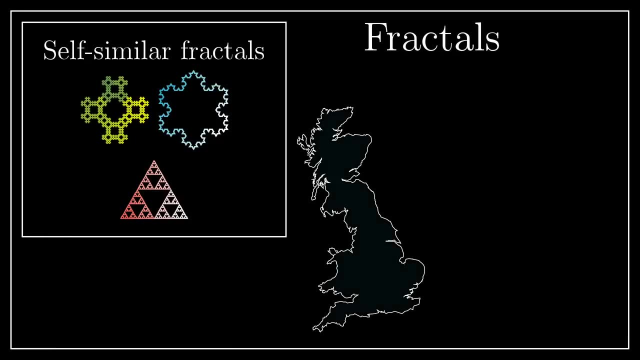 And don't get me wrong: self-similar shapes are definitely beautiful and they're a good toy model for what fractals really are. But Mandelbrot had a much broader conception in mind, one motivated not by beauty but more by a pragmatic desire to model nature in a way that actually captures roughness. 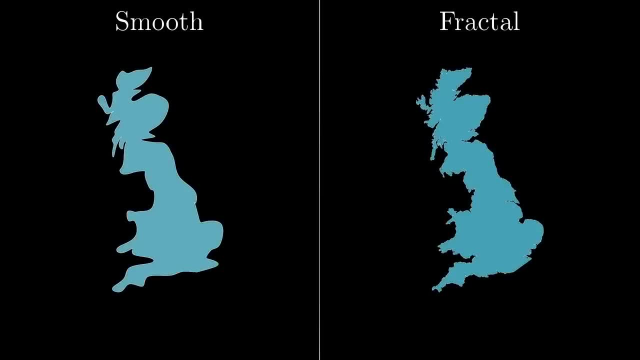 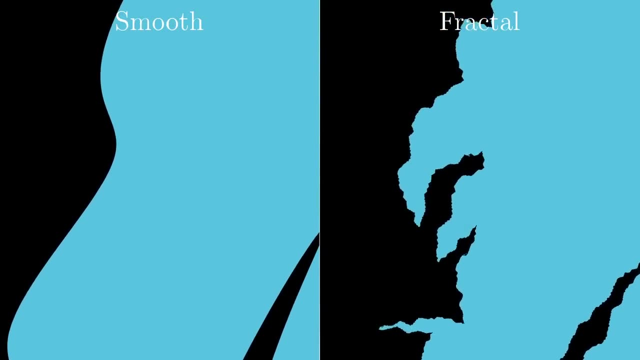 In some ways, fractal geometry is a rebellion against calculus, whose central assumption is that things tend to look smooth if you zoom in far enough. But Mandelbrot saw this as overly idealized, or at least needlessly idealized, resulting in models that neglect. 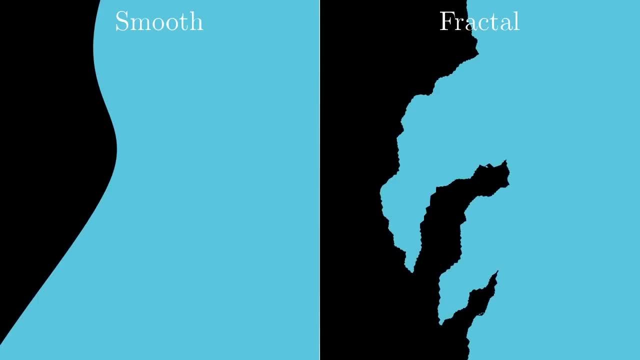 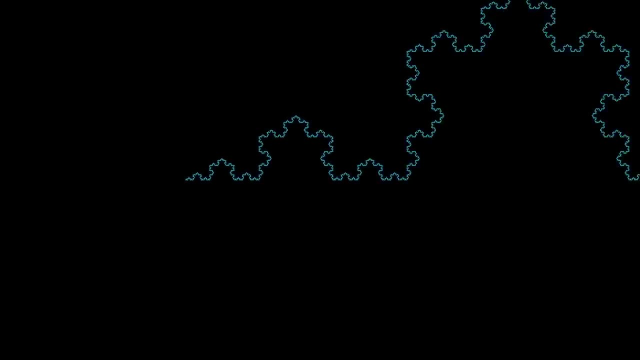 the finer details of the thing they're actually modeling which can matter. What he observed is that self-similar shapes give a basis for modeling the regularity in some forms of roughness, But the popular perception that fractals only include perfectly self-similar. 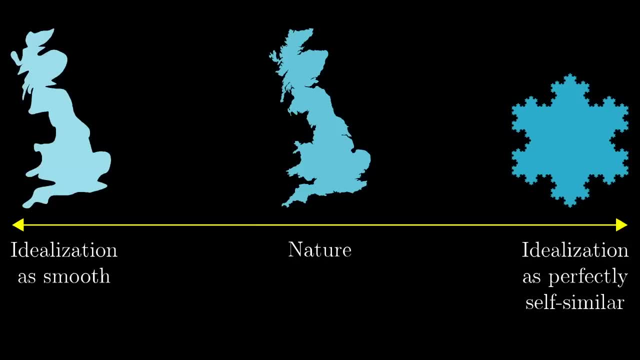 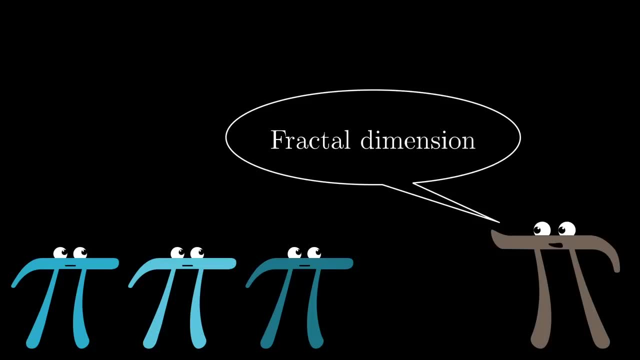 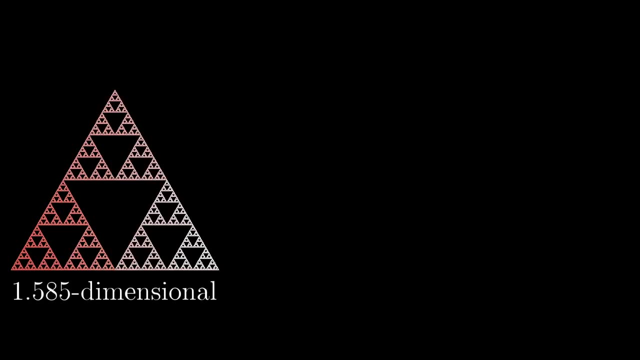 shapes is another over-idealization, one that ironically goes against the pragmatic spirit of fractal geometry's origins. The real definition of fractals has to do with this idea of fractal dimension, the main topic of this video. There is a sense, a certain way to define the word dimension, in which the Sierpinski 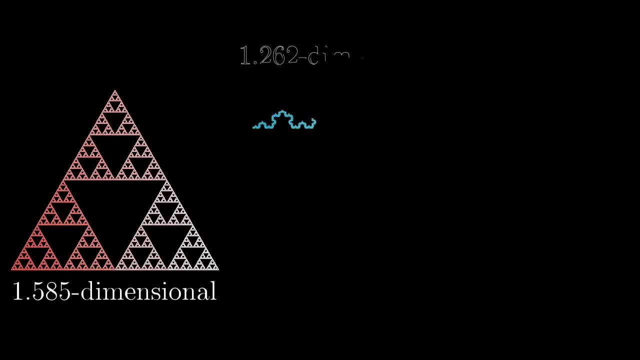 triangle is approximately 1.585 dimensional, that the von Koch curve is approximately 1.262 dimensional. the coastline of Britain turns out to be around 1.21 dimensional and in general it's possible to have shapes whose dimension is any positive real number not. 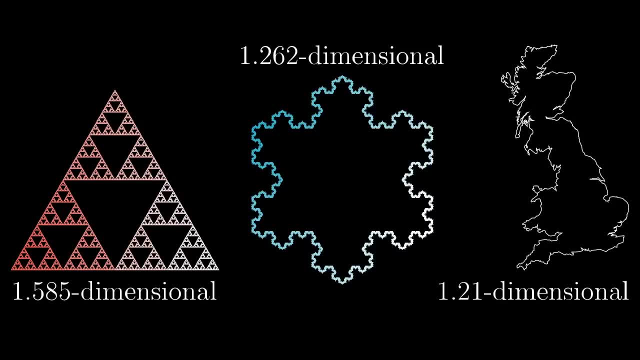 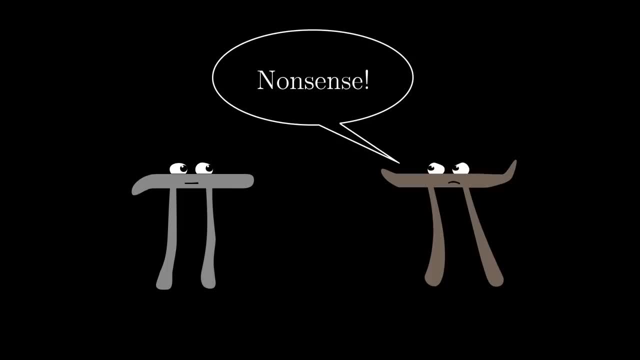 just whole numbers. I think when I first heard someone reference fractional dimension like this, I just thought it was nonsense, right? I mean, mathematicians are clearly just making stuff up. Dimension is something that usually only makes sense for natural numbers, right? A line is one-dimensional. 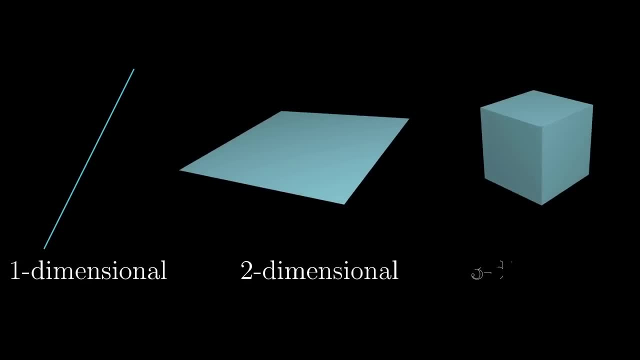 a plane is two-dimensional, the space that we live in is three-dimensional, and so on. And in fact any linear algebra student who just learned the formal definition of dimension in that context would agree. it only makes sense for counting numbers. 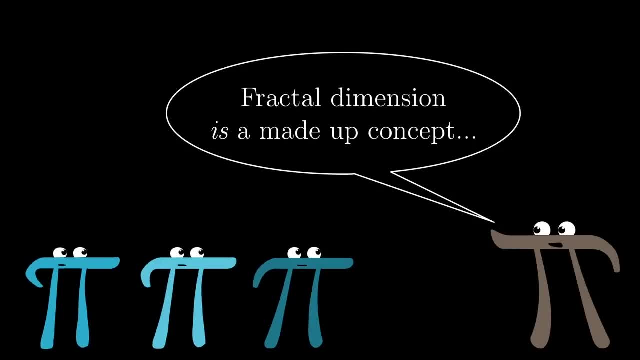 And, of course, the idea of fractal dimension is just made up. I mean, this is math, everything's made up, But the question is whether or not it's true, Whether or not it turns out to be a useful construct for modeling the world. 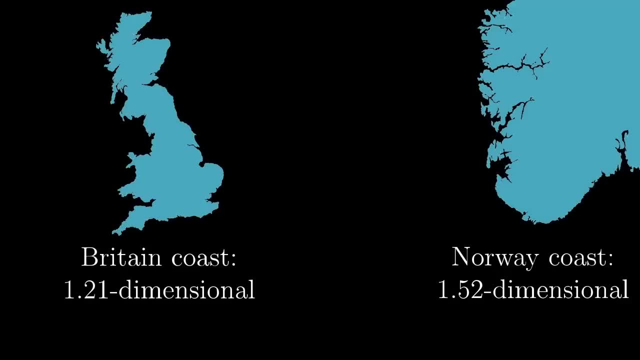 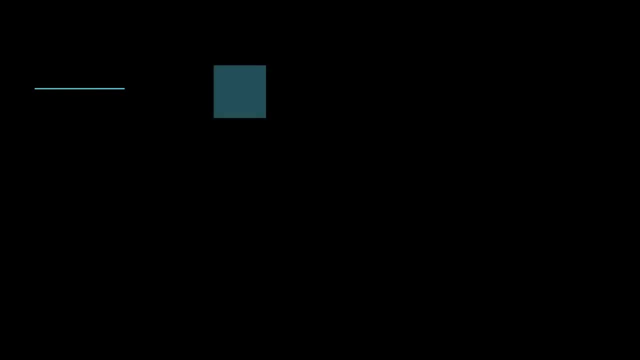 And I think you'll agree, once you learn how fractal dimension is defined, it's something that you start seeing almost everywhere you look. It actually helps to start the discussion here by only looking at perfectly self-similar shapes. In fact, I'm going to start with four shapes, the first three of which aren't even fractals. 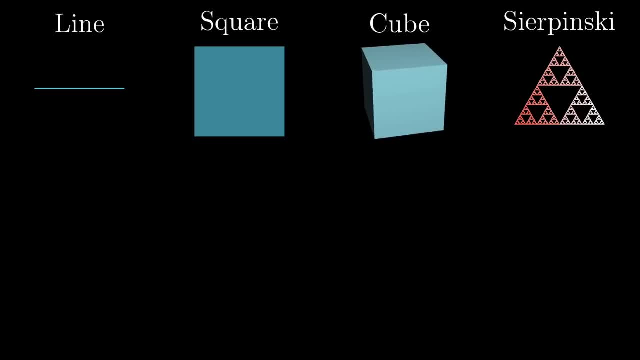 A line, a square, a cube and a Sierpinski triangle. All of these shapes are self-similar. A square can be broken down into two smaller lines, each of which is a perfect copy of the original, just scaled down by a half. 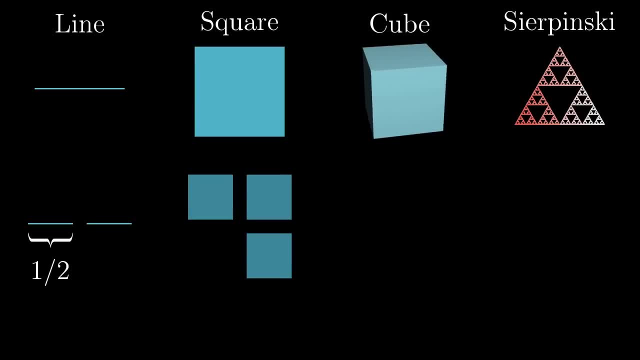 A square can be broken down into four smaller squares, each of which is a perfect copy of the original, just scaled down by a half. Likewise, a cube can be broken down into eight smaller cubes. again, each one is a scaled-down version by one half. 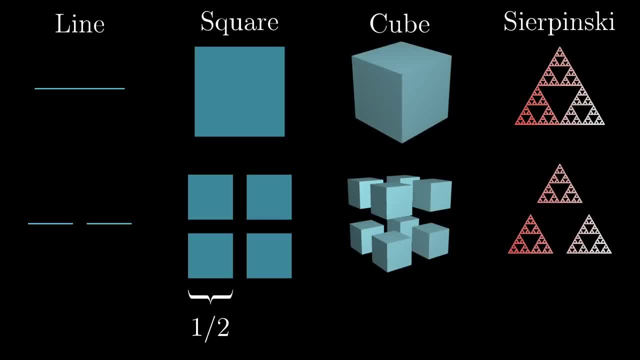 And the core characteristic of the Sierpinski triangle is that it's made of three smaller copies of itself, and the length of the side of one of those smaller copies is one-half the side length of the original. Now it's fun to compare how we measure these things. 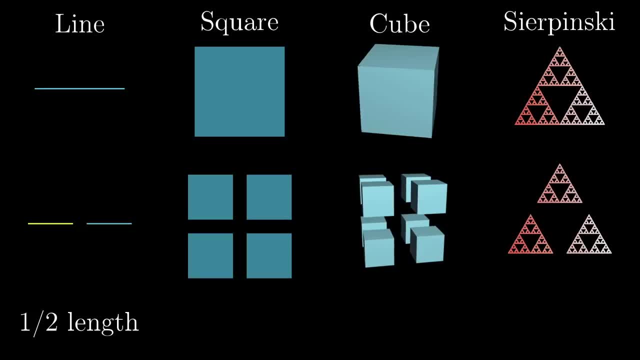 We'd say that the smaller line is one-half the length of the original line, the smaller square is one-quarter the area of the original square, the smaller cube is one-eighth the volume of the original cube and that smaller Sierpinski triangle. 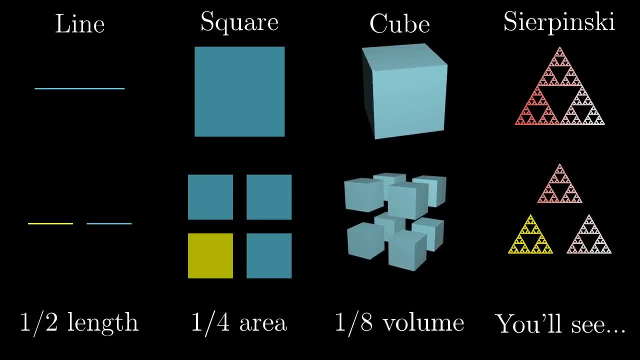 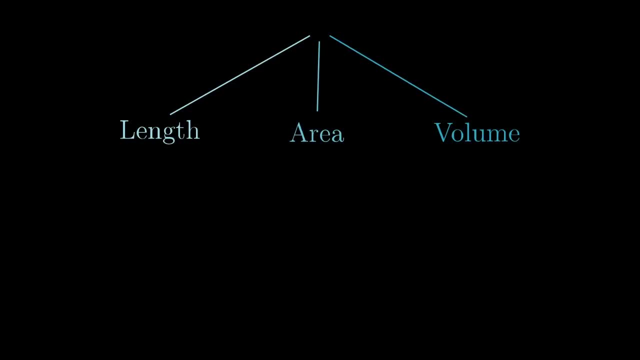 Well, we'll talk about how to measure that in just a moment. What I want is a word that generalizes the idea of length, area and volume, but that I can apply to all of those shapes and, more Typically, in math the word that you'd use for this is measure, but I think it might. 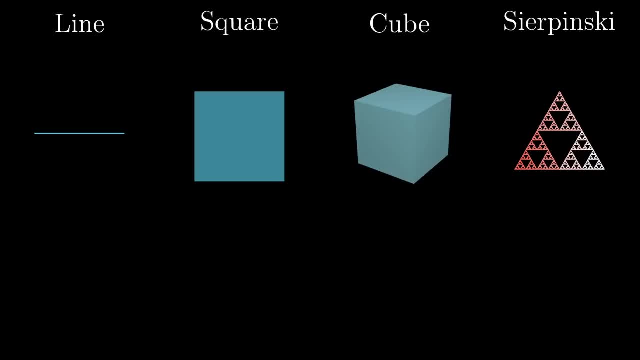 be more intuitive to talk about mass, As in. imagine that each of these shapes is made out of metal: a thin wire, a flat sheet, a solid cube and some kind of Sierpinski mesh. Fractal dimension has everything to do with understanding how the mass of these shapes 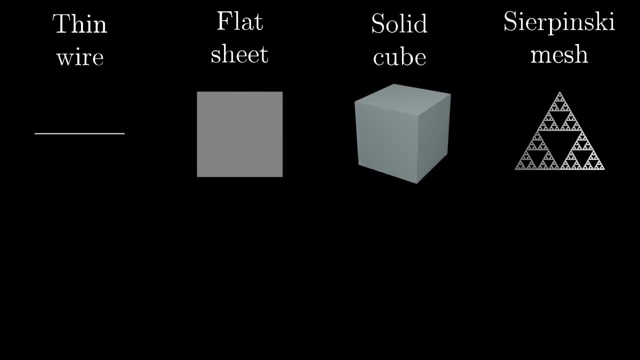 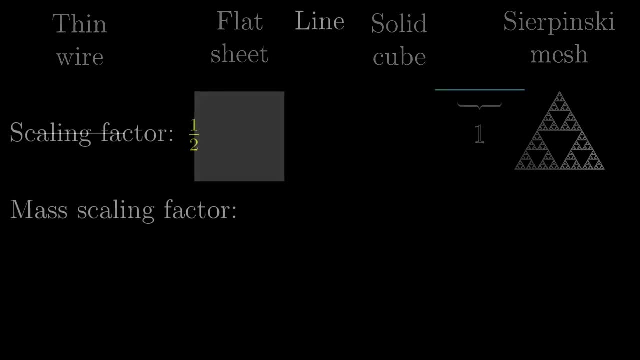 changes as you scale them. The benefit of starting the discussion with self-similar shapes is that it gives us a nice, clear-cut way to compare masses. When you scale down that line by one-half, the mass is also scaled down by one-half. 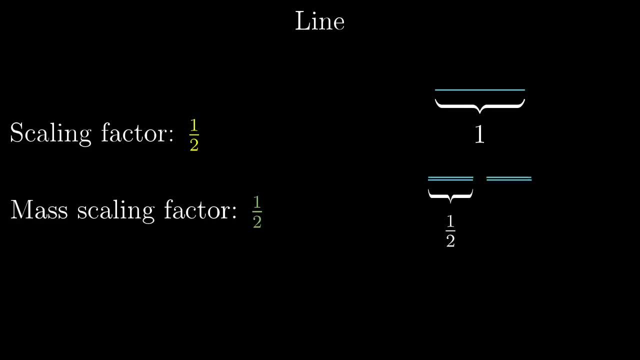 which you can viscerally see, because it takes two copies of that smaller one to form the whole. When you scale down a square by one-half, its mass is scaled down by one-fourth, where, again, you can see this by piecing together four of the smaller copies to get the original. 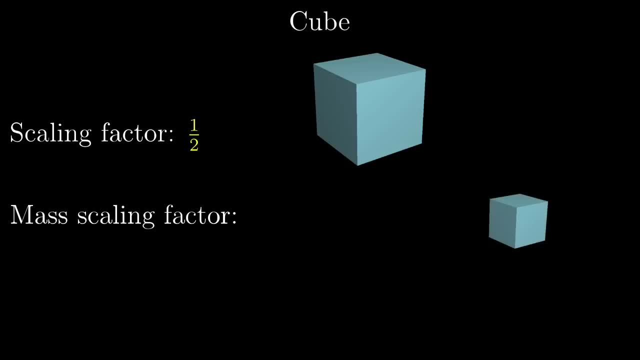 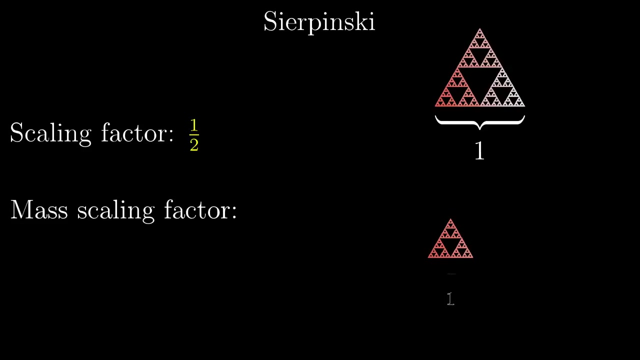 Likewise, when you scale down that cube by one-half, the mass is scaled down by one-eighth or one-half cubed. This is because it takes eight copies of that smaller cube to rebuild the original. And when you scale down the Sierpinski triangle by a factor of a half, wouldn't you agree? 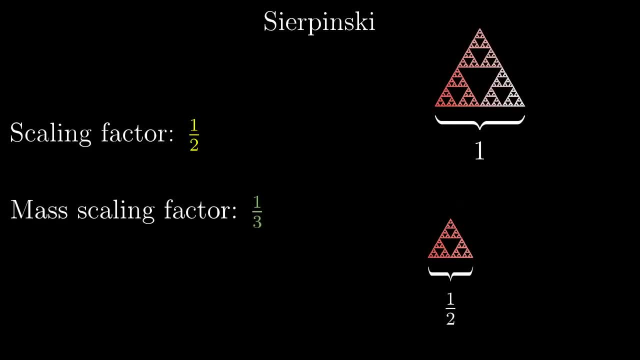 that it makes sense to say that its mass goes down by a factor of one-third. I mean it takes exactly three of those smaller ones to form the original. But notice that for the line, the square and the cube, the factor by which the mass 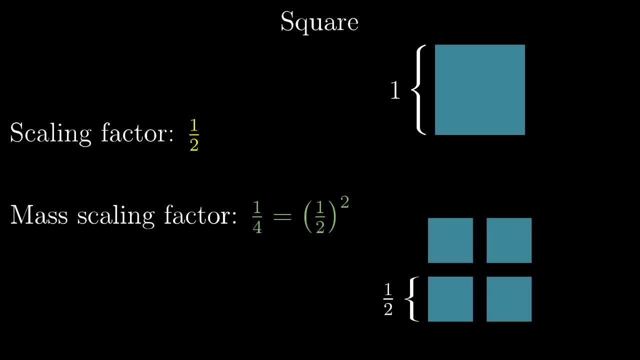 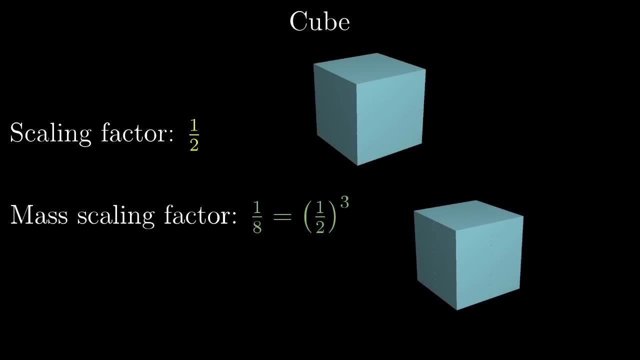 changed is this nice, clean integer power of one-half. In fact, that exponent is the mass of the cube, It's not the square or the cube, It's the cube, It's the dimension of each shape. And what's more, you could say that what it means for a shape to be, for example, two-dimensional. 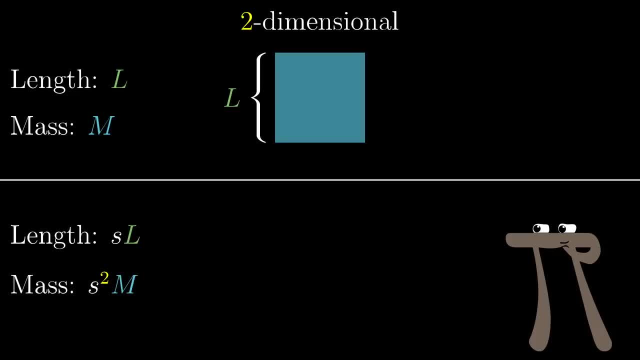 what puts the two in two-dimensional is that when you scale it by some factor, its mass is scaled by that factor raised to the second power. And maybe what it means for a shape to be three-dimensional is that when you scale it by some factor, the mass is scaled by that factor raised to the second power. 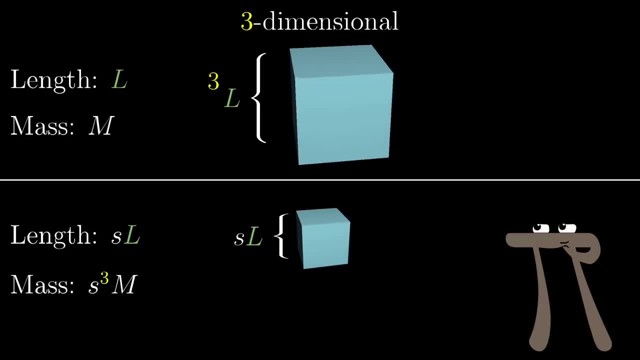 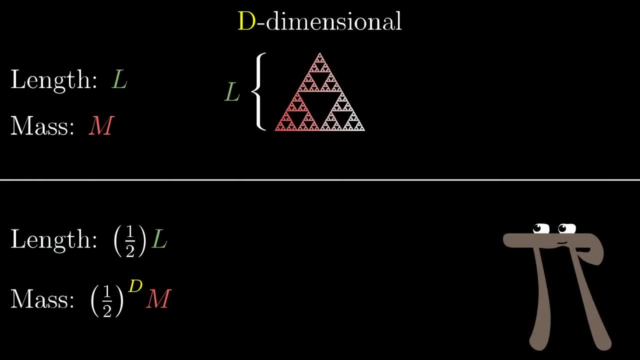 The mass is scaled by the third power of that factor. So if this is our conception of dimension, what should the dimensionality of a Sierpinski triangle be? You'd want to say that when you scale it down by a factor of one-half, its mass goes down. 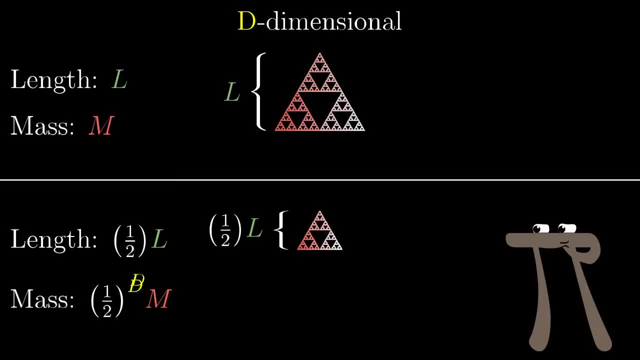 by one-half to the power of. well, whatever its dimension is, And because it's self-similar, we know that we want its mass to go down by a factor of one-third. So what's the number d? Well, that's the same as asking 2 to the. what equals 3, the quintessential type of question. 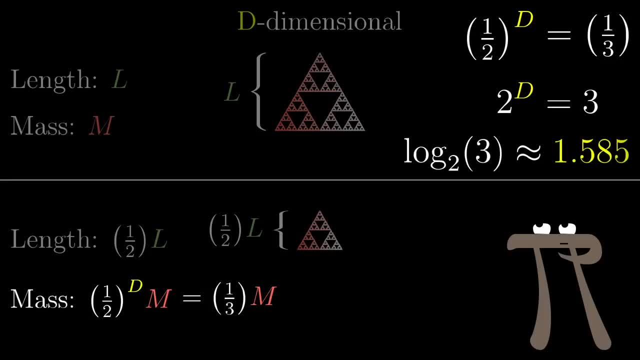 that logarithms are meant to answer. And when you go and plug in log base 2 of 3 to a calculator, what you'll find is that it's about 1.585.. So in this way, the Sierpinski triangle is not one-dimensional, even though you could. 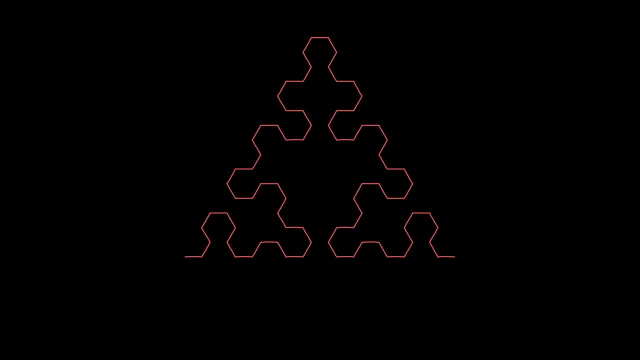 define a curve that passes through all its points, and nor is it two-dimensional, even though it lives in the plane. Instead, it's 1.585-dimensional, And if you want to describe its mass, neither length nor area seem like the fitting notions. 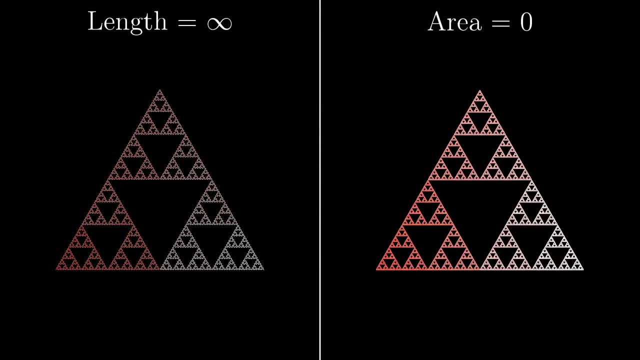 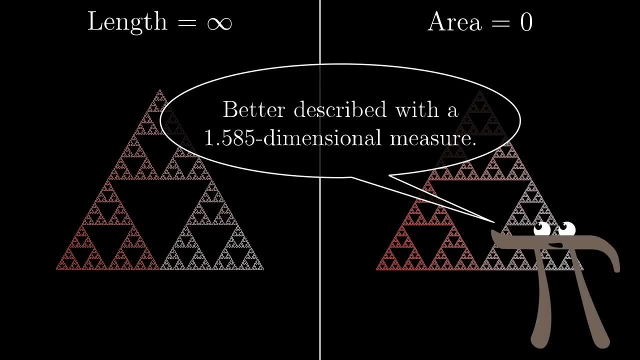 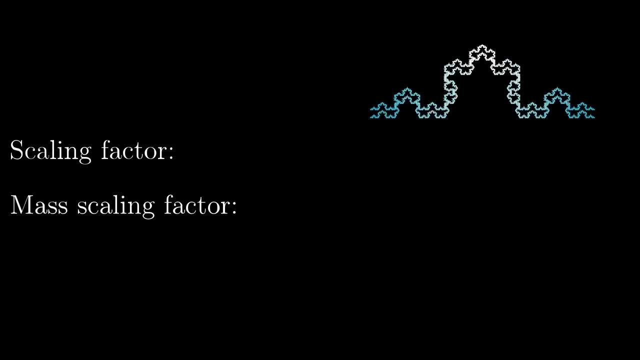 If you tried, its length would turn out to be infinite and its area would turn out to be zero. Instead, what you want is: whatever. the 1.585-dimensional analog of length is Here. let's look at another self-similar fractal, the von Koch curve. 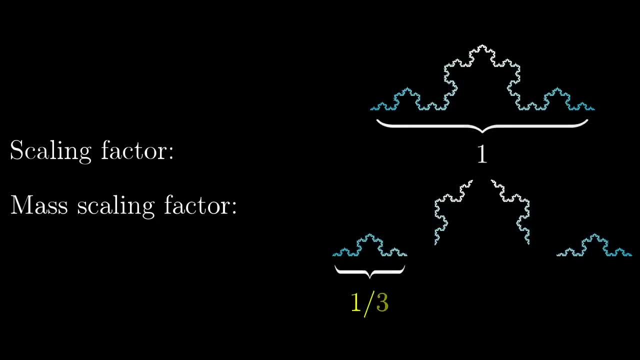 This one is composed of four smaller, identical copies of itself, Each of which is a self-similar fractal, Each of which is a copy of the original, scaled down by one-third. So the scaling factor is one-third and the mass has gone down by a factor of one-fourth. 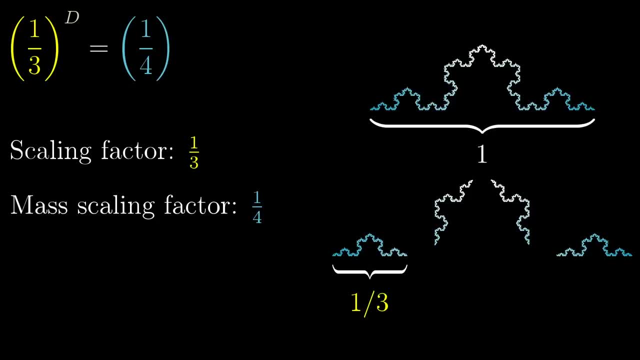 So that means the dimension should be some number d, so that when we raise one-third to the power of d it gives us one-fourth. Well, that's the same as saying 3 to the, what equals 4, so you can go and plug in to a calculator. 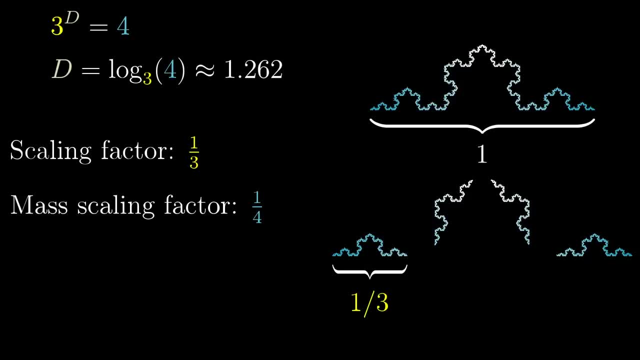 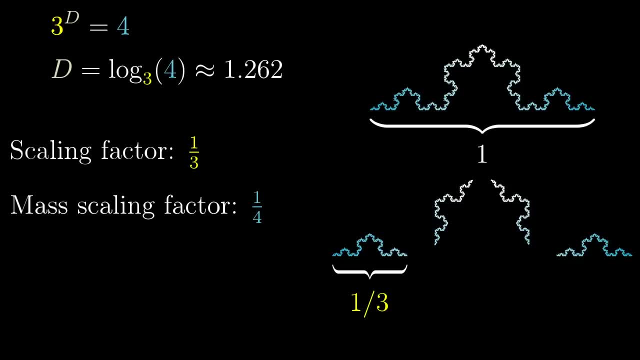 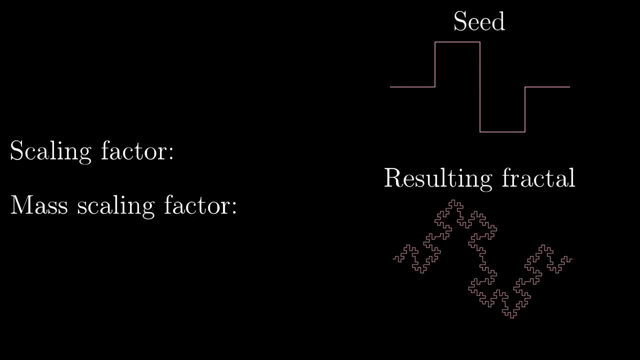 So in a sense it's about 1.262.. The von Koch curve is one-point-two-six-two dimensional. Here's another fun one. This is kind of the right-angled version of the Koch curve. It's built up of eight scaled-down copies of itself, where the scaling factor is one-fourth. 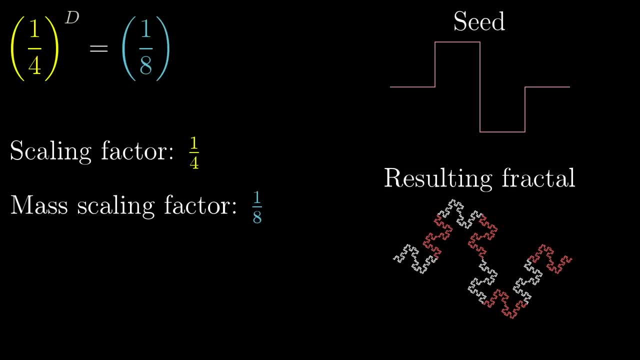 So if you want to know its dimension, it should be some number d such that one-fourth to the power of d equals one-eighth the factor by which the mass just decreased. And in this case the value we want is log base 4 of 8, and that's exactly 3 halves. 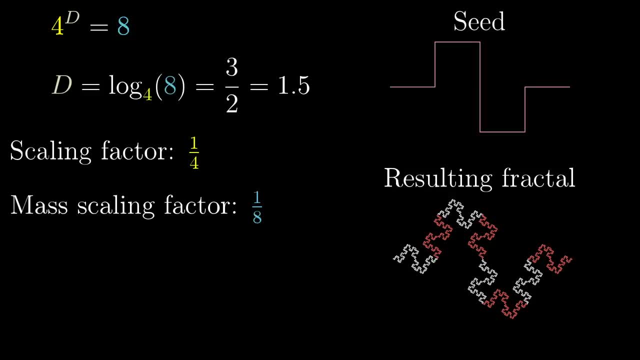 So evidently this fractal is precisely 1.5-dimensional. Does that kind of make sense? It's weird, but it's all just about scaling and comparing masses while you scale, And what I've described so far, everything up to this point, is what you might call self-similarity. 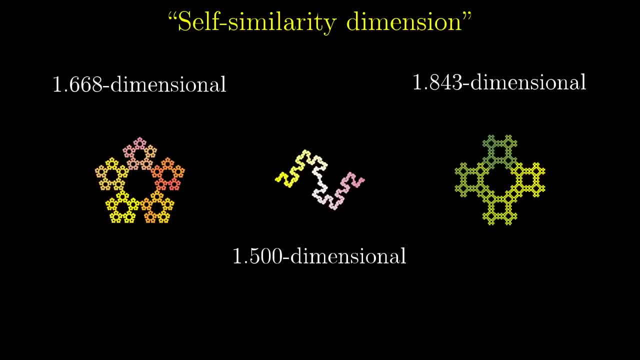 dimension. You can do a good job making the idea of fractional dimensions seem at least somewhat reasonable. but there's a problem. It's not really a general notion. When we were reasoning about how a mass's shape should change, it relied on the self-similarity. 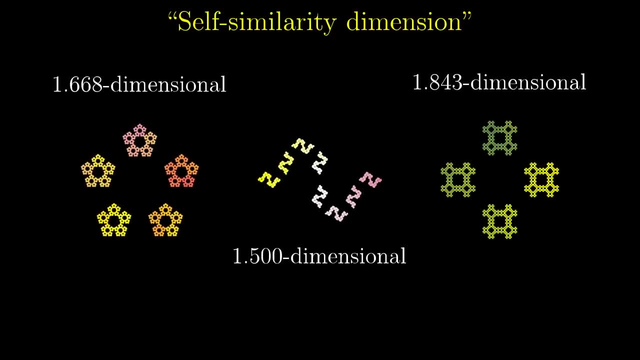 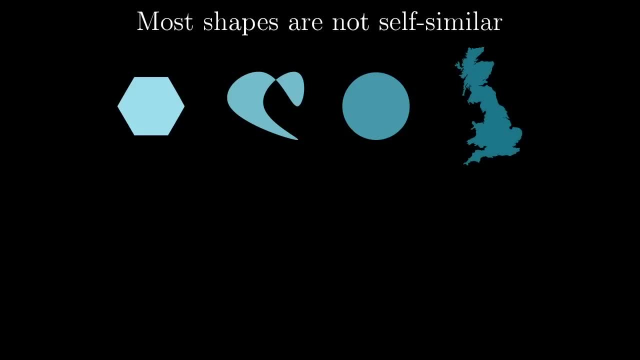 of the shapes, that you could build them up from smaller copies of themselves. But that seems unnecessarily restrictive. After all, most 2-dimensional shapes are not at all self-similar. Consider the disc: the interior of a circle. We know that's 2-dimensional. 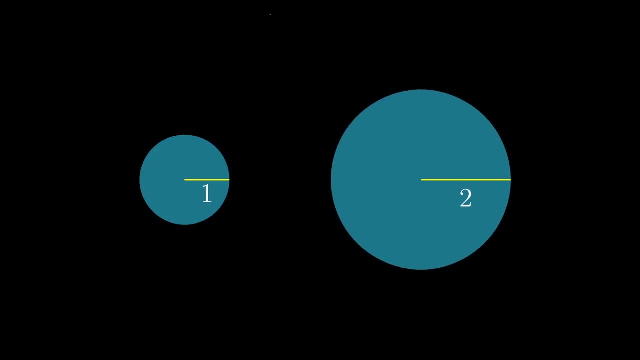 And you could say that this is because we know it's 2-dimensional. And you could say that this is because we know it's 2-dimensional, But when you scale it up by a factor of 2, its mass proportional to the area gets scaled. 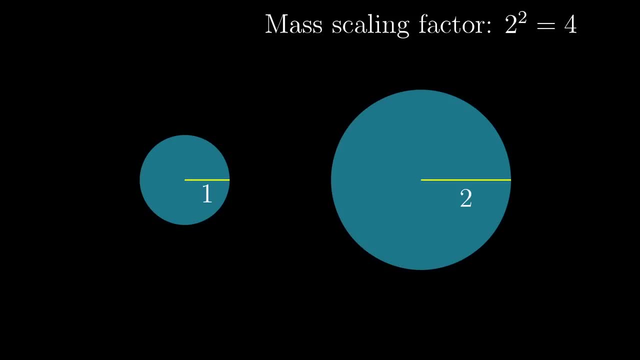 by the square of that factor, in this case 4.. But it's not like there's some way to piece together 4 copies of that smaller circle to rebuild the original. So how do we know that that bigger disc is exactly 4 times the mass of the original? 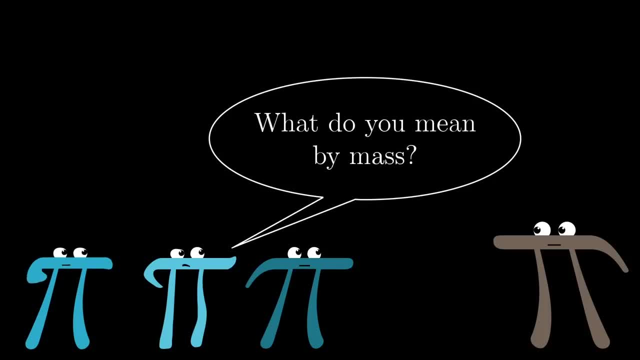 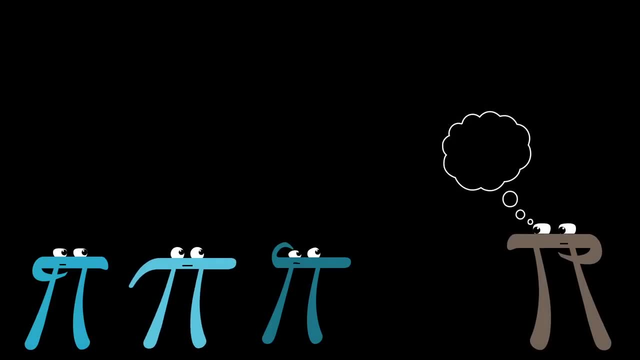 Answering. that requires a way to make this idea of mass a little more mathematically rigorous, Since we're not dealing with physical objects made of matter, are we? We're not dealing with physical objects made of matter, are we? We're dealing with purely geometric ones living in an abstract space. 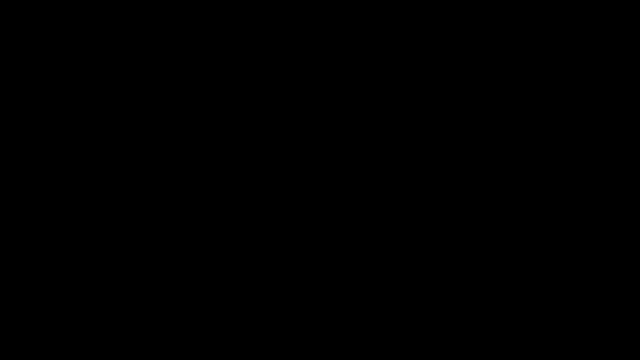 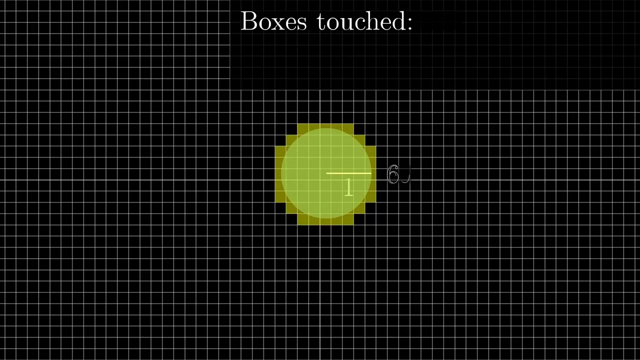 And there's a couple ways to think about this, but here's a common one: Cover the plane with a grid and highlight all of the grid squares that are touching the disc and now count how many there are. In the back of our minds, we already know that a disc is 2-dimensional and the number 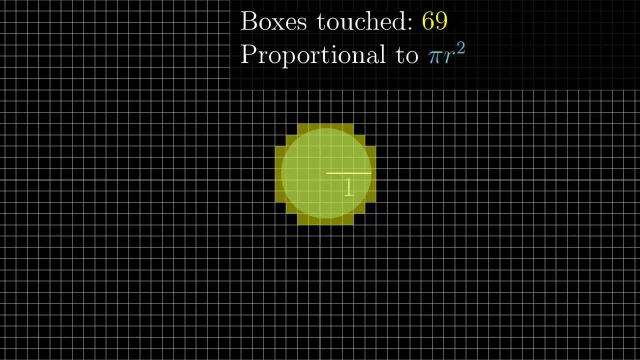 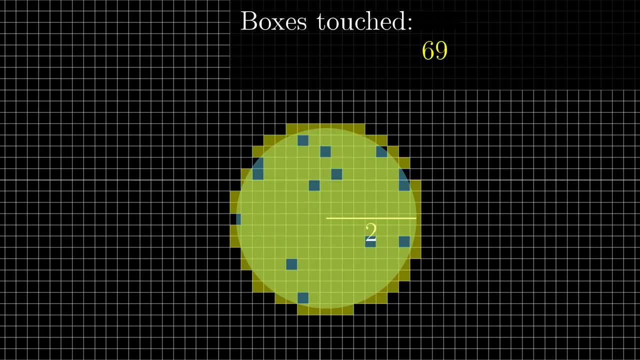 of grid squares that it touches should be proportional to its area. A clever way to verify this empirically is to scale up that disc by some factor like 2, and count how many grid squares touch this new scaled-up version. What you should find is that that number has increased approximately in proportion to the 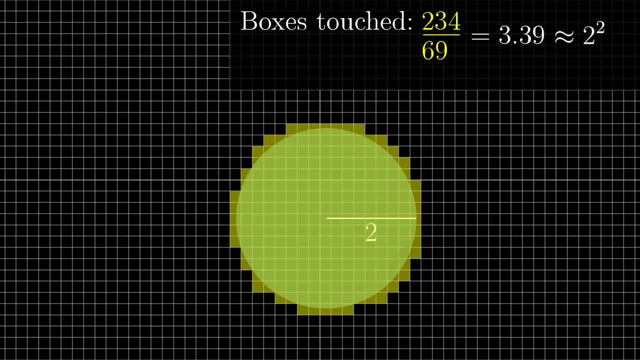 square of our scaling factor, which in this case means about 4 times as many boxes. Well, admittedly, what's on the screen here might not look that convincing, but it's just because the grid is really coarse. If, instead, you took a much finer grid, one that more tightly captures the intent, we're 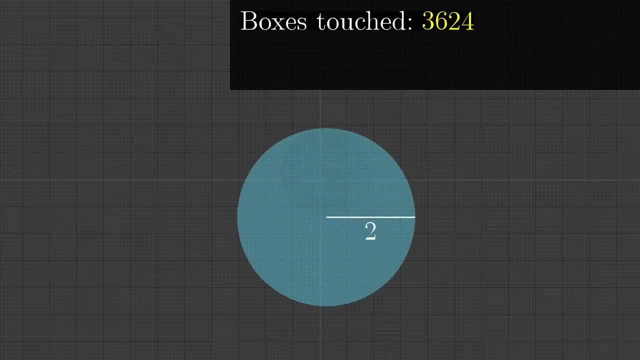 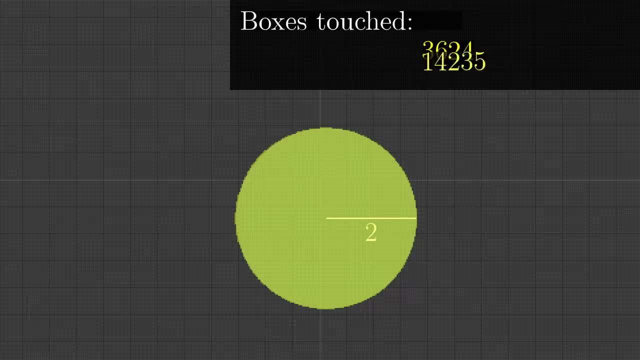 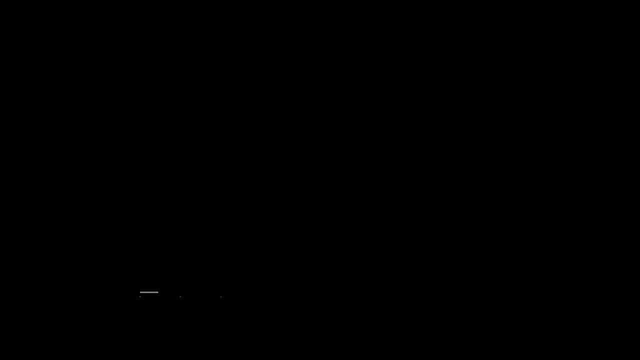 We're going to measure the size of the circle, So the number of boxes touched when you scale the disc by a factor of 2…. jakie van siO should shine through more clearly If you were to plot that scaling factor judgement ف compared to the number of boxes Horizontal. 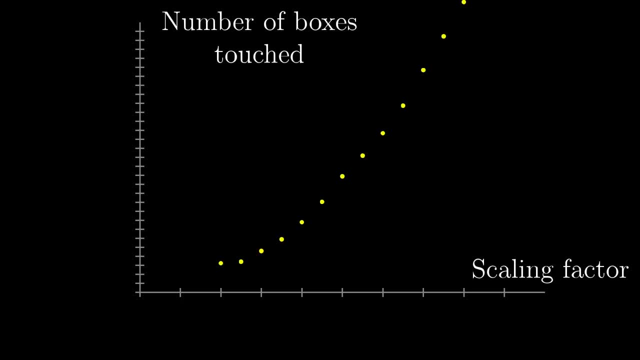 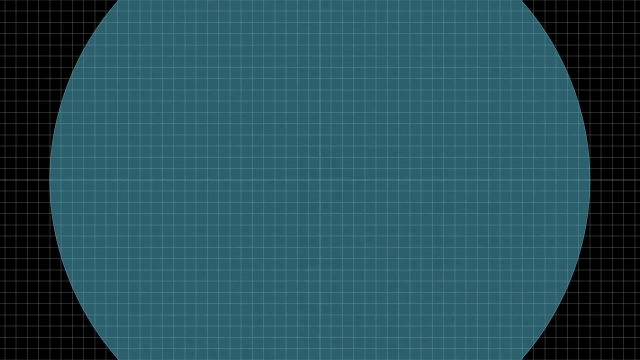 ter, your data should very closely fit a perfect parabola, since the number of boxes touched is roughly proportional to the square of the scaling factor от 50.. For larger and larger scaling values, which is actually equivalent to just looking at a finer grid, that data is going to more perfectly fit that parabola. 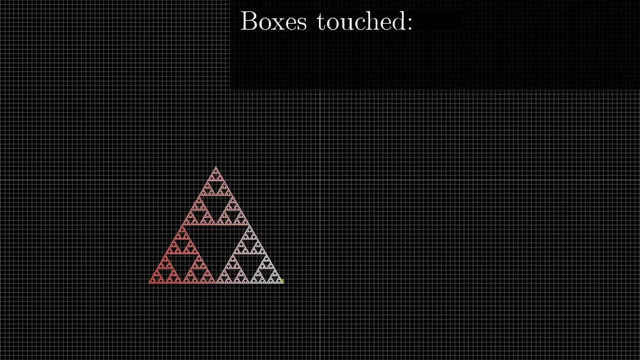 Now getting back to fractals. let's play this game with the Sierpinski triangle, counting how many boxes are touching points in that shape. How would you imagine that number compares to scaling up the triangle by a factor of two and counting the new number of boxes touched? 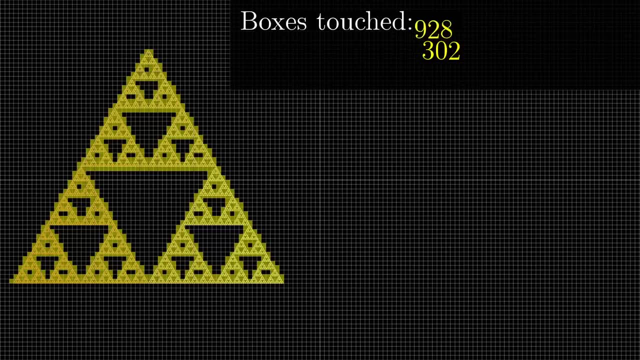 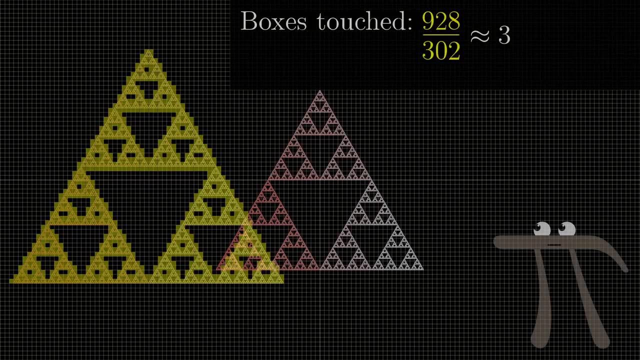 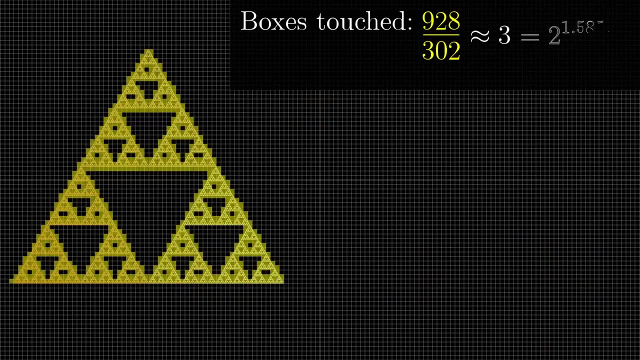 Well, the proportion of boxes touched by the big one to the number of boxes touched by the small one should be about three. After all, that bigger version is just built up of three copies of the smaller version. You could also think about this as two, raised to the dimension of the fractal. 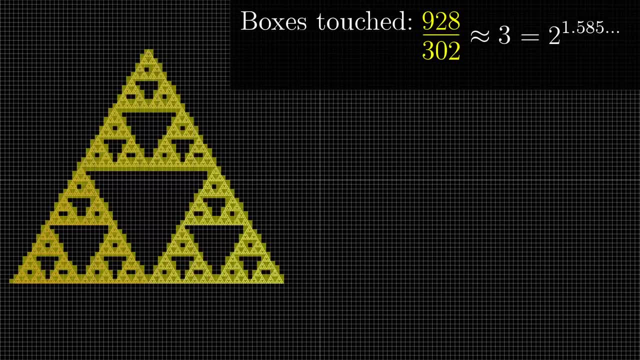 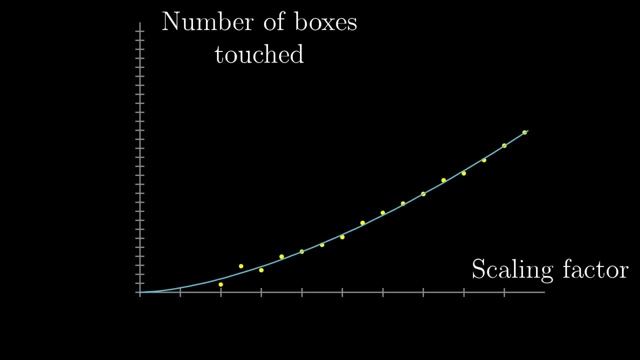 which we just saw is about 1.585.. And so if you were to go and plot the scaling factor in this case against the number of boxes touched by the Sierpinski triangle, the data would closely fit a curve with the shape of y equals x to the power 1.585,. 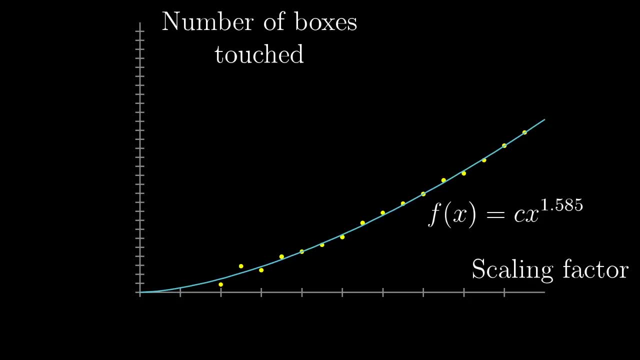 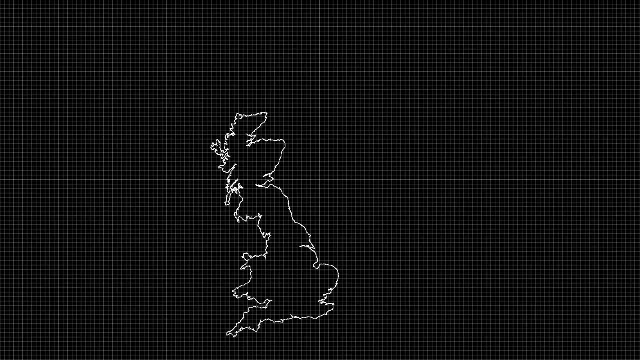 just multiplied by some proportionality constant. But, importantly, the whole reason that I'm talking about this is that we can play the same game with non-self-similar shapes that still have some kind of roughness, And the classic example here is the coastline of Britain. 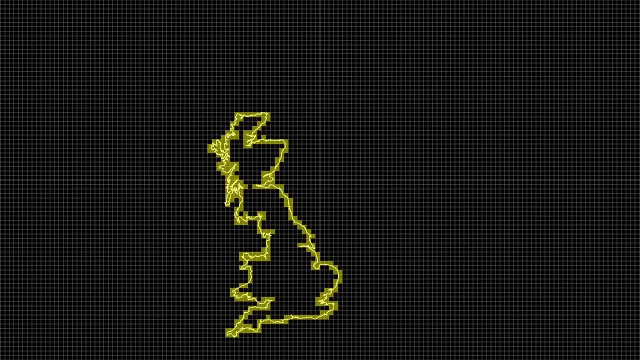 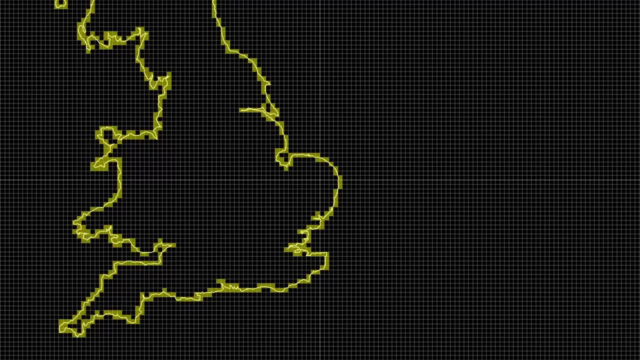 If you plop that coastline into the plane and count how many boxes are touching it, and then scale it by some amount and count how many boxes are touching that new scaled version, what you'd find is that the number of boxes touching the coastline increases approximately. 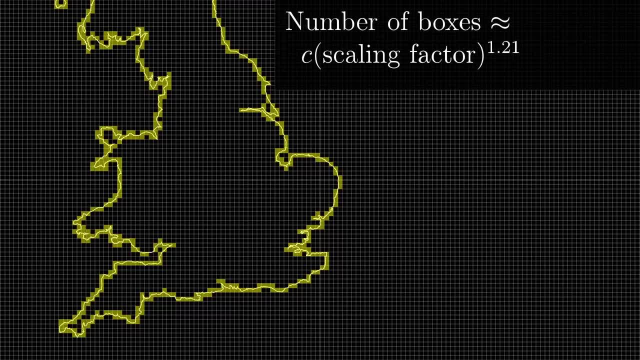 in proportion to the scaling factor raised to the power of 1.21.. Here it's kind of fun to think about how you would actually compute that number empirically, As in. imagine I give you some shape and you're a savvy programmer, how would you find this number? 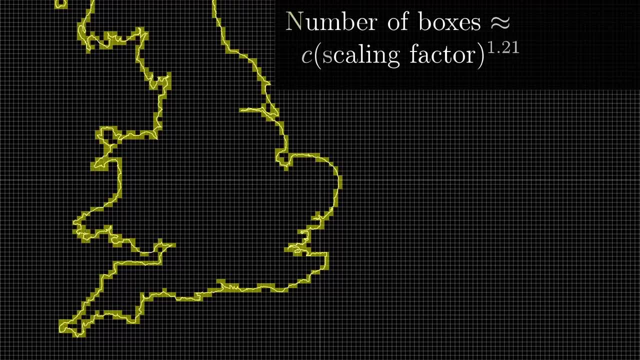 So what I'm saying here is that if you scale this shape by some factor, which I'll call s, the number of boxes touching that shape should equal some constant multiplied by that scaling factor. raised to whatever the dimension is the value that we're looking for. 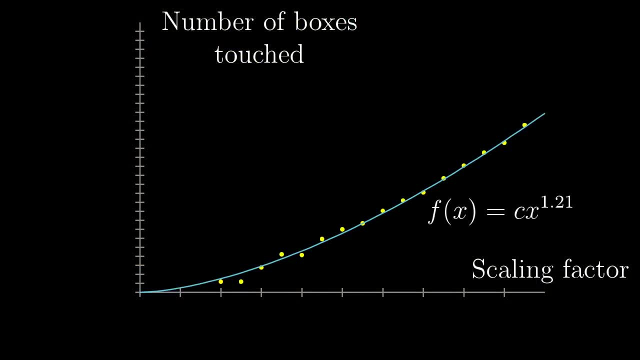 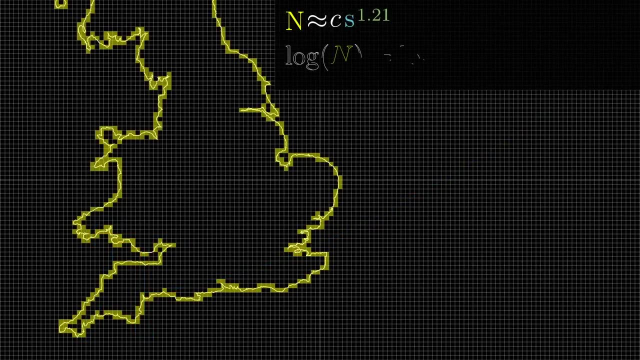 Now, if you have some data plot that closely fits a curve that looks like the input raised to some power, it can be hard to see exactly what that power should be. So a common trick is to take the logarithm of both sides. That way the dimension is going to drop down from the exponent. 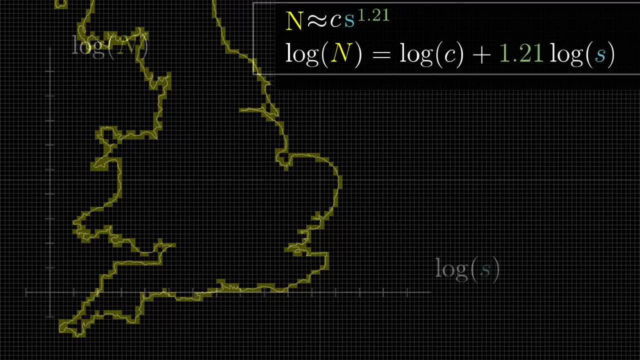 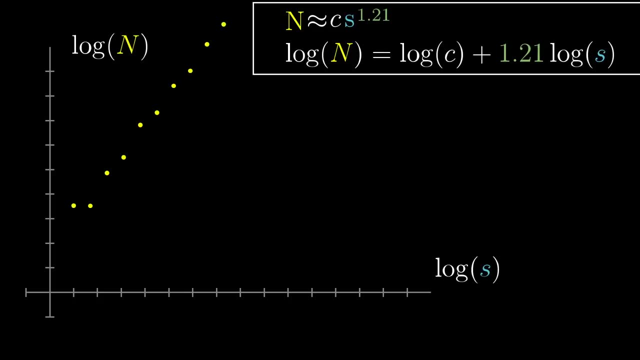 and we'll have a nice clean, linear relationship. What this suggests is that if you were to plot the log of the scaling factor against the log of the number of boxes touching the coastline, the relationship should look like a line, and that line should have a slope equal to the dimension. 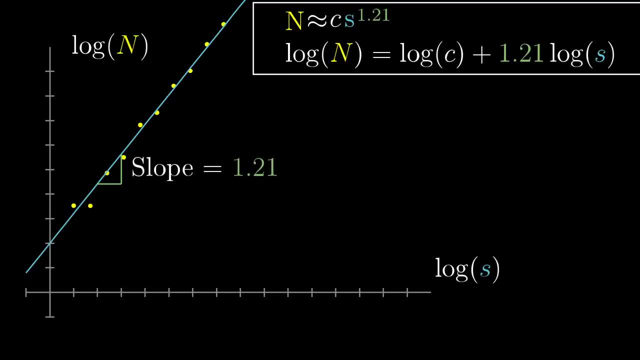 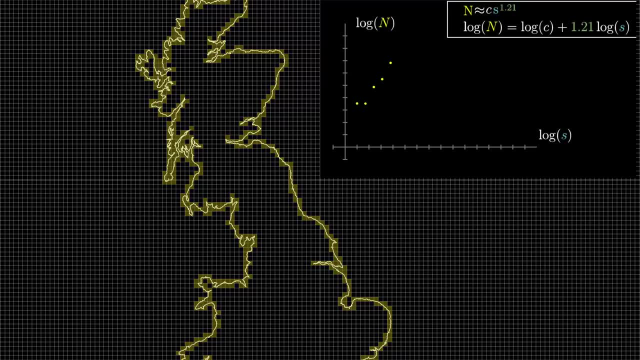 So what that means is that if you tried out a whole bunch of scaling factors, counted the number of boxes touching the coast in each instant and then plotted the points on the log-log plot, you could then do some kind of linear regression to find the best fit line to your 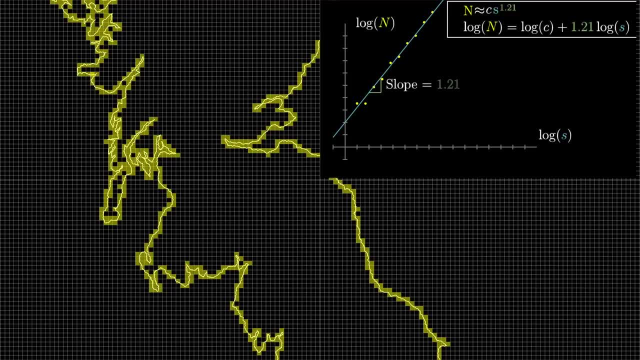 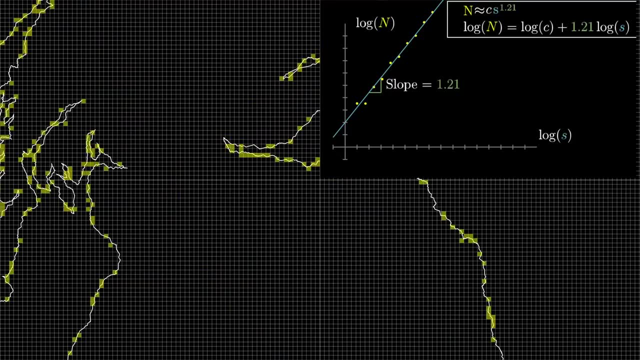 data set And when you look at the slope of that line, that tells you the empirical measurement for the dimension of what you're examining. I just think that makes this idea of fractal dimension so much more real and visceral compared to abstract, artificially perfect shapes. 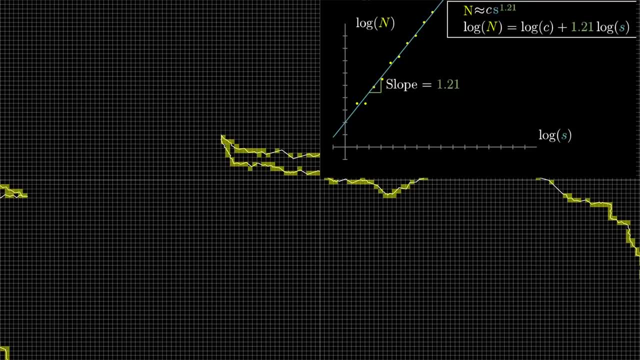 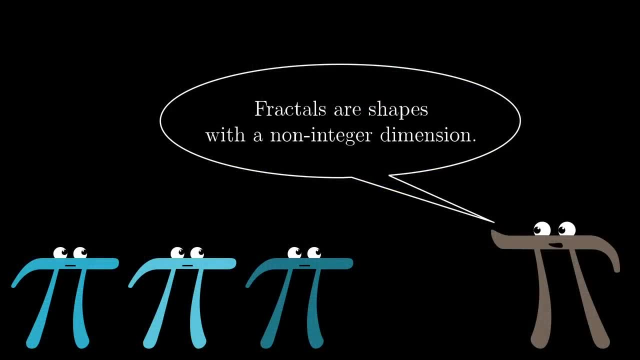 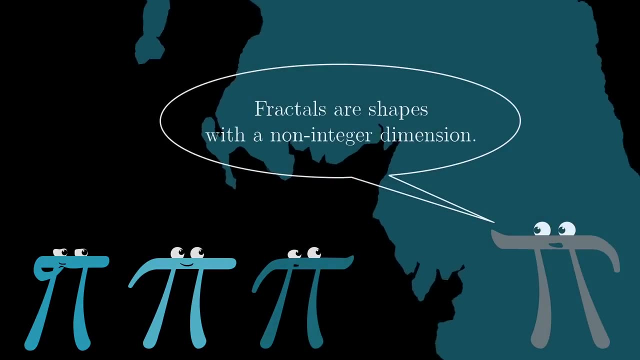 And once you're comfortable thinking about dimension like this, you, my friend, have become ready to hear the definition of a fractal. Essentially, fractals are shapes whose dimension is not an integer but instead some fractional amount. What's cool about that is that it's a quantitative way to say that they're shapes. 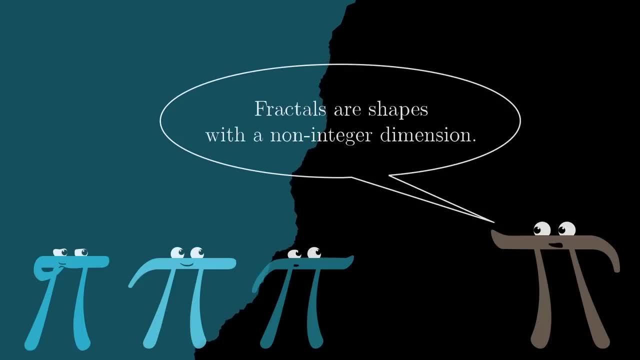 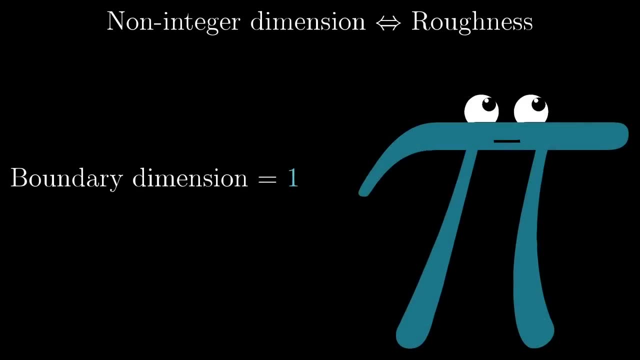 that are rough and that they stay rough even as you zoom in. Technically there's a slightly more accurate definition and I've included it in the video description, but this idea here of a non-integer dimension almost entirely captures the idea of 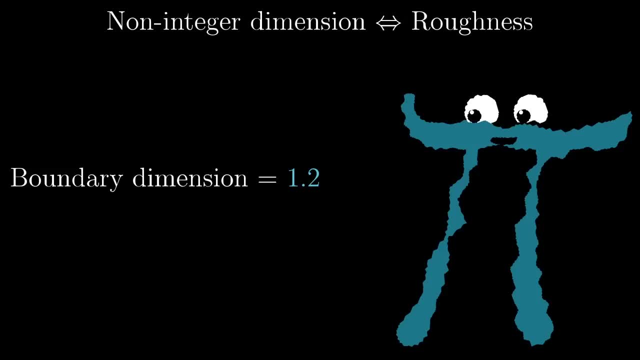 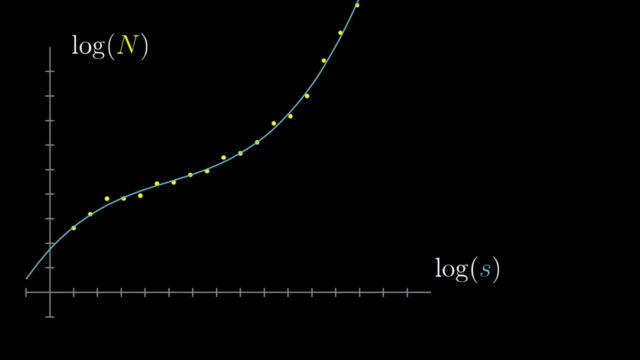 roughness that we're going for. There is one nuance, though, that I haven't brought up yet, but it's worth pointing out, which is that this dimension, at least as I've described it so far using the box-counting method- 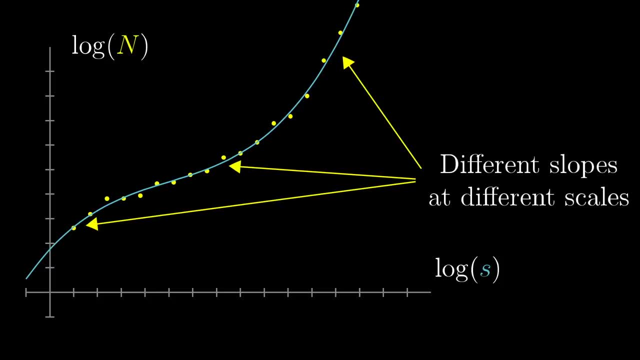 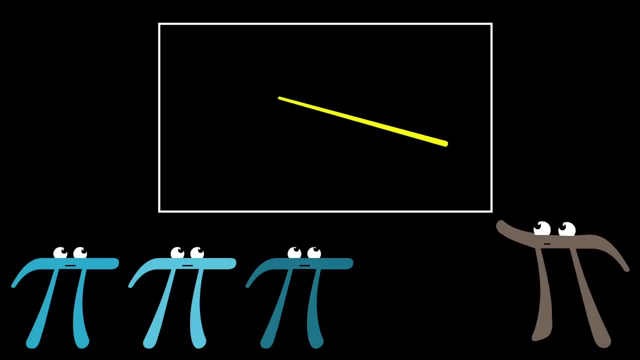 can sometimes change based on how far zoomed in you are. For example, here's a shape sitting in three dimensions which, at a distance, looks like a line In 3D. by the way, when you do a box counting, you have a 3D grid full of little cubes instead of. 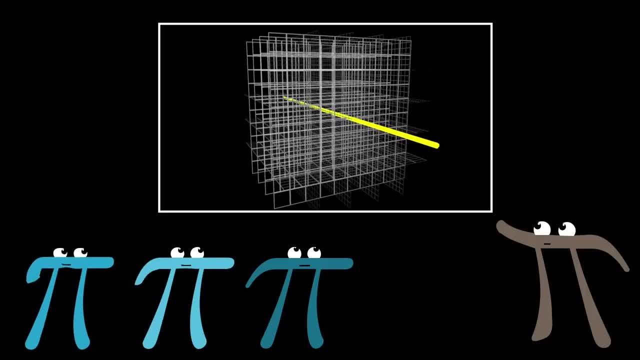 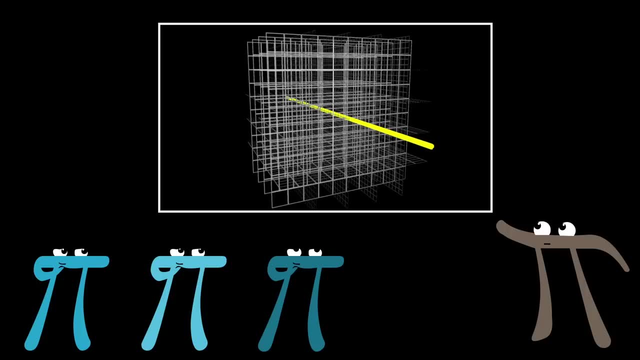 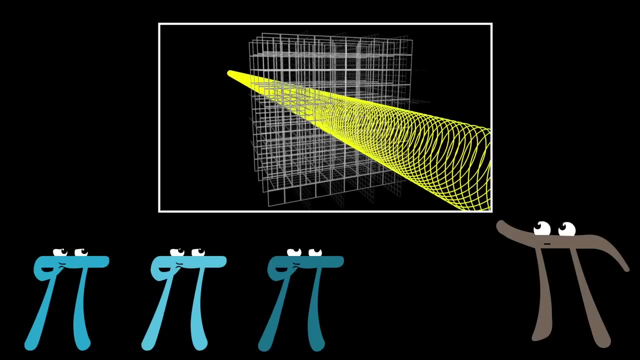 little squares, but it works the same way. At this scale, where the shape's thickness is smaller than the size of the boxes, it looks one-dimensional, meaning the number of boxes it touches is proportional to its length, But when you scale it up it starts behaving a lot more like a tube. 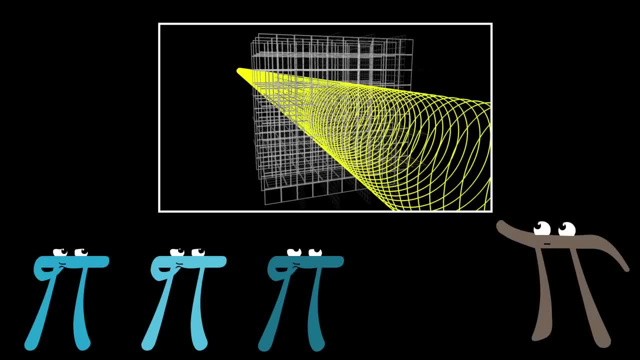 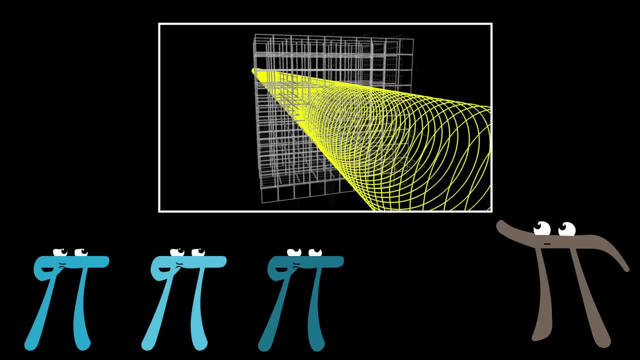 touching the boxes on the surface of that tube, and so it'll look two-dimensional, with the number of boxes touched being proportional to the square of the scaling factor. But it's not really a tube. it's made of these rapidly winding little curves. 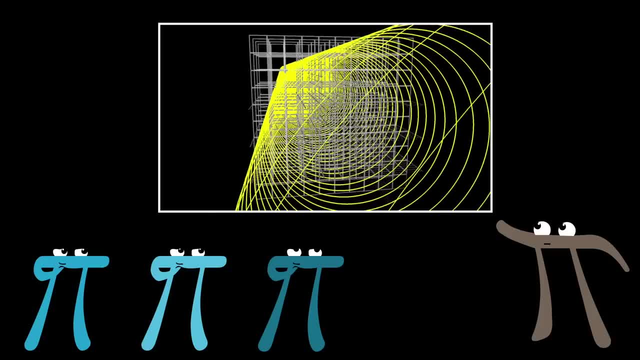 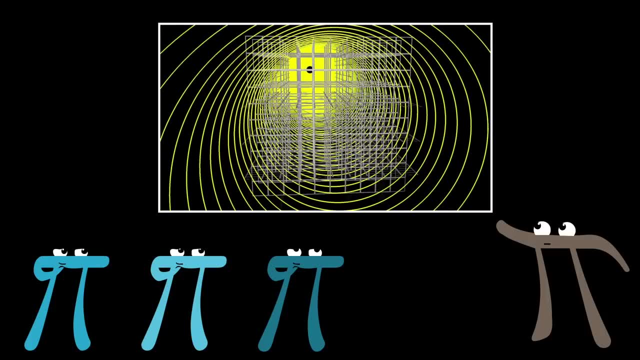 So once you scale it up even more, to the point where the boxes can pick up on the details of those curves, it looks one-dimensional again, with the number of boxes touched scaling directly in proportion to the dimensions, to the scaling constant, So actually assigning a number to a shape for its. 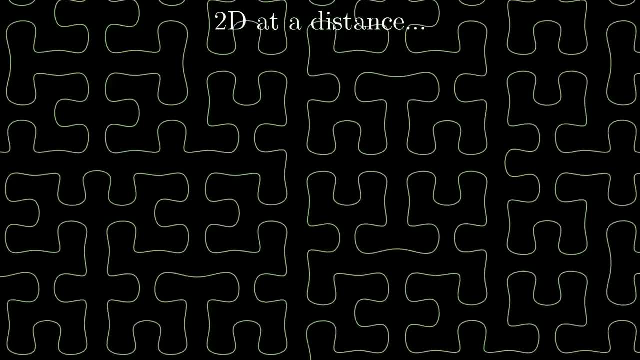 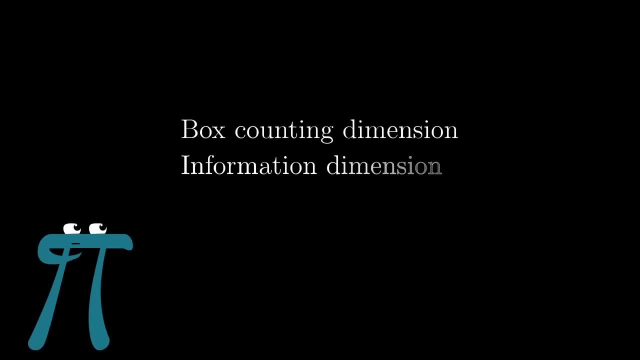 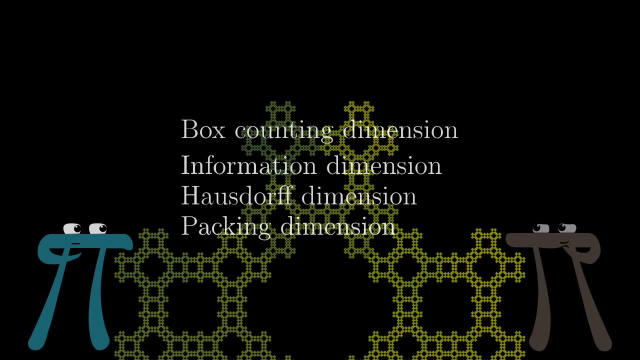 dimension can be tricky, and it leaves room for differing definitions and differing conventions. In a pure math setting, there are indeed numerous definitions for dimension, but all of them focus on what the limit of this dimension is at closer and closer zoom levels. You can think of that in terms of 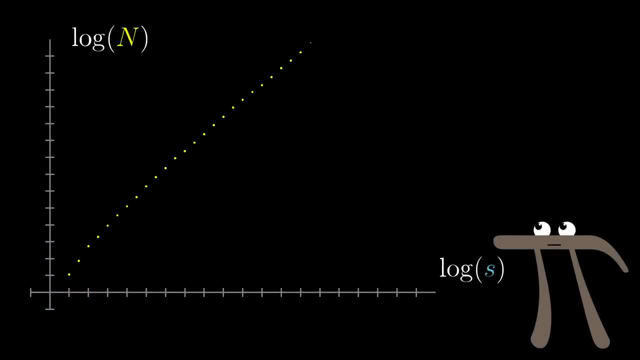 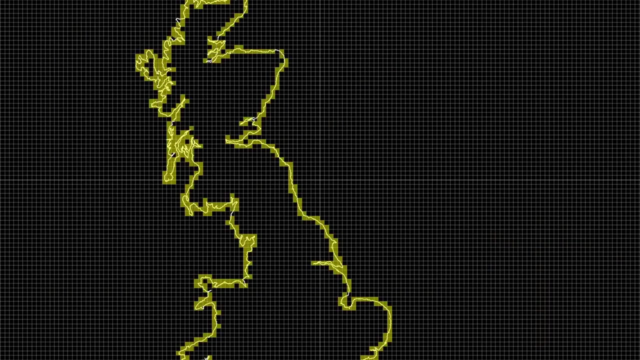 the plot as the limit of this slope as you move farther and farther to the right. So for a purely geometric shape to be a genuine fractal, it has to continue looking rough, even as you zoom in infinitely far. But in a more applied setting, like looking at the coastline of Britain, it doesn't really make sense to 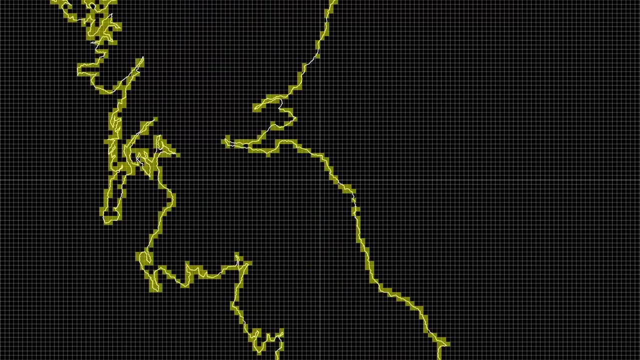 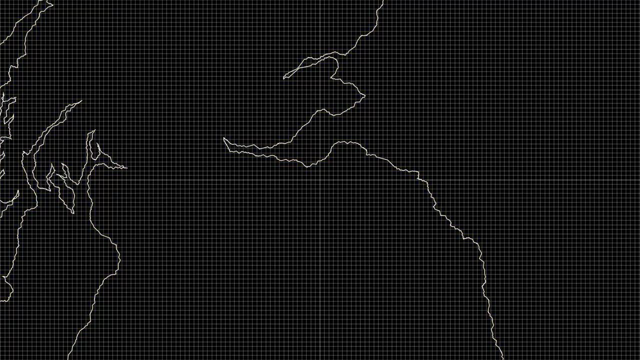 talk about the limit as you zoom in more and more. I mean, at some point you'd just be hitting atoms. Instead, what you do is you look at a sufficiently wide range of scales, from very zoomed out up to the bottom of the scale, and then zoom in. 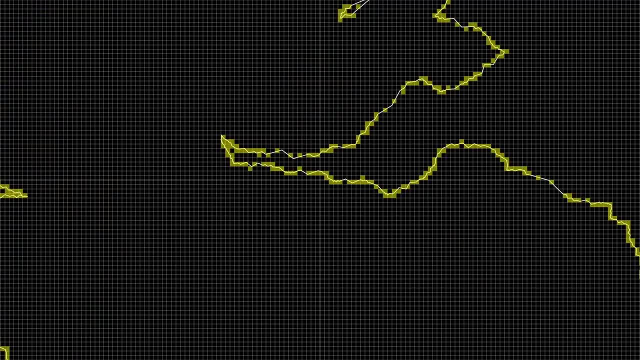 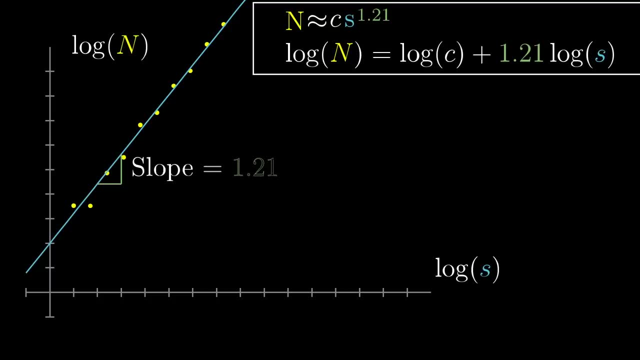 up to very zoomed in and compute the dimension at each one, And in this more applied setting, a shape is typically considered to be a fractal only when the measured dimension stays approximately constant even across multiple different scales. For example, the coastline of Britain doesn't just look 1.21. 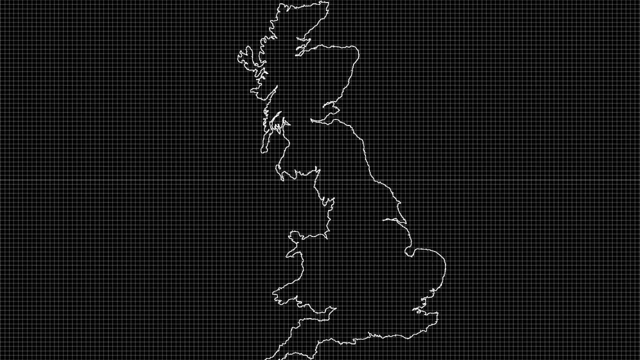 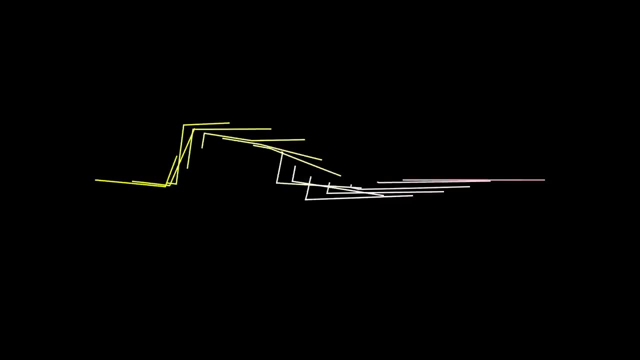 dimensional at a distance. Even if you zoom in by a factor of a thousand, the level of roughness is still around 1.21.. That right there, is the sense in which many shapes from nature actually are self-sustaining. Perfectly self-similar shapes do play an important role in fractal geometry. What they give us. 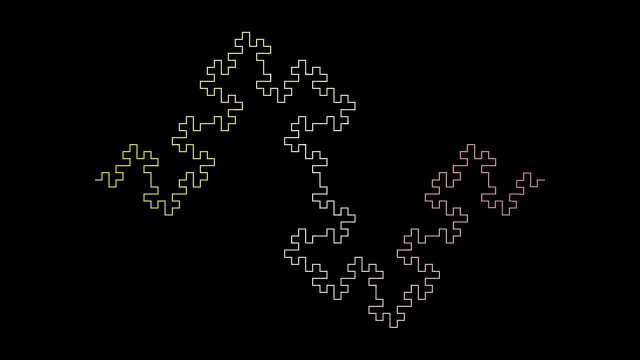 are simple-to-describe, low-information examples of this phenomenon of roughness, roughness that persists at many different scales and at arbitrarily close scales. It gives us the primitive tools for modeling these fractal phenomena, But I think it's also important. 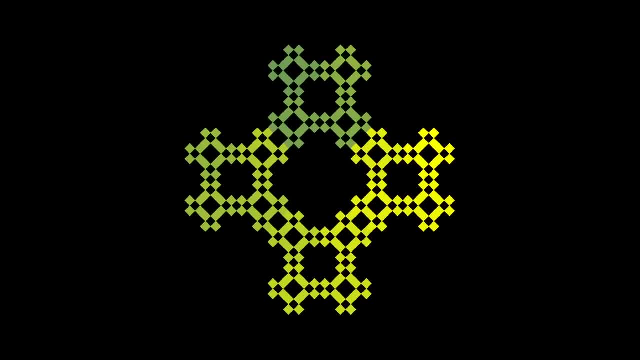 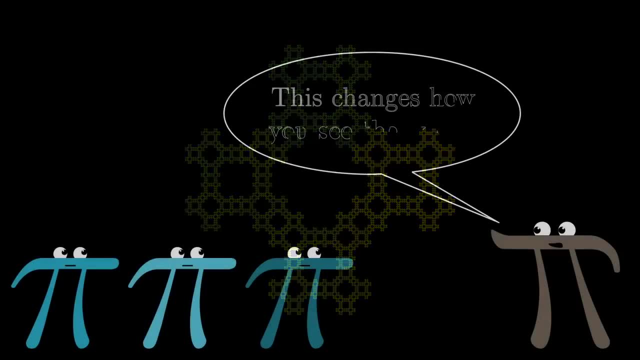 not to view them as the prototypical example of fractals, since fractals in general actually have a lot more character to them. I really do think that this is one of those ideas where, once you learn it, it makes you start looking at the world completely differently. What this number?